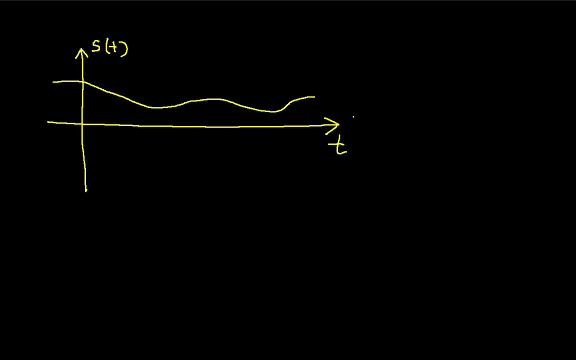 it is a sensor output as a function of time, Perhaps it is music. It's basically something that might change as a function of time And, in general, I would like to be able to know exactly what this signal is, because I need to measure. 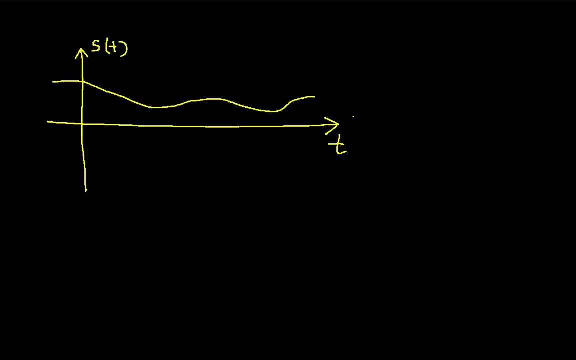 something exactly, or I would like my music to sound beautiful and distortion-free, But oftentimes in the real world I'll have either extrinsic or intrinsic noise, And so, instead of having my signal, I end up with something that looks sort of like this: 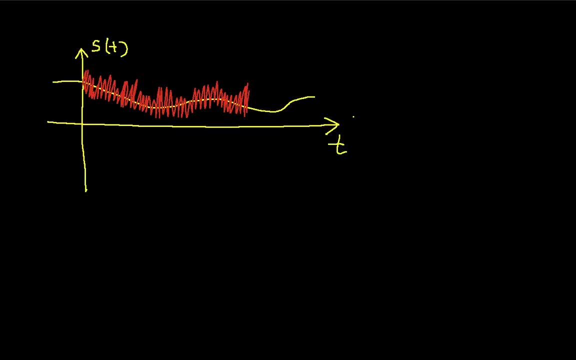 So instead of having a nice exact waveform, I have a waveform that wiggles around a lot, and sometimes it deviates from my signal enough to be quite noticeable And it just basically makes it hard to figure out what my signal was. This happens almost universally. 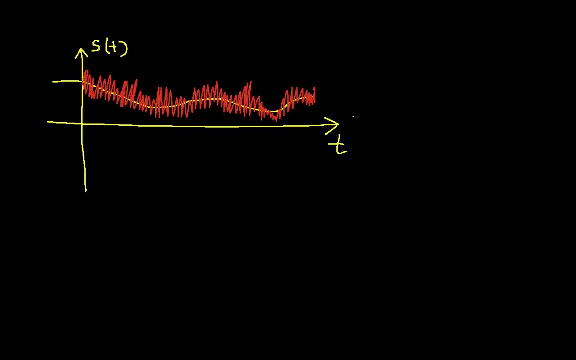 It turns out that this sort of phenomenon is one of the limiting factors in a communication system. The fact that there is noise added to signals makes it impossible to transmit infinite amounts of information over a finite bandwidth communication system. And that's essentially true due to noise. 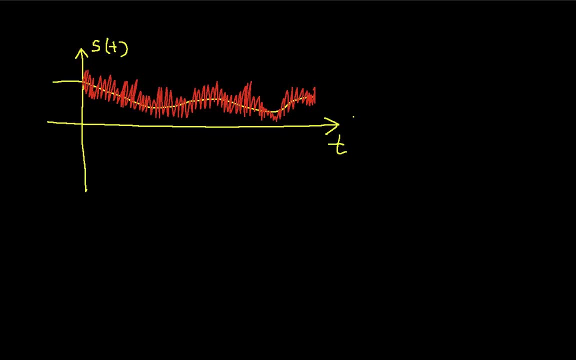 So what we'd like to do is we would like to be able to characterize the relative strength of the signal and the noise, And we do this through what's called a signal-to-noise ratio, SNR. S stands for signal, N stands for noise, R stands for ratio. 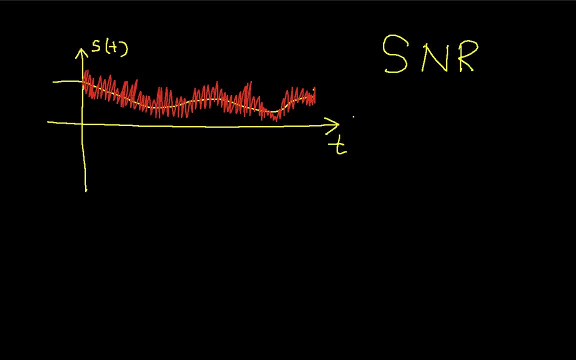 There are several different types of signal-to-noise ratios that we use. One is called a power signal-to-noise ratio, where you would have the signal or the average signal power in volts squared divided by the average noise power, again in volts squared. 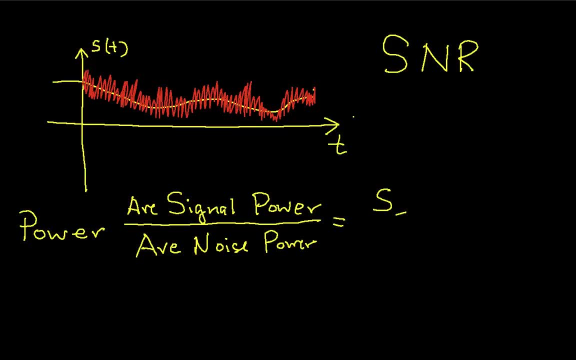 And typically we'll give the average signal power the symbol S and the average noise power the symbol N, So you can represent that as S over N. Now, sometimes we want to talk about our noise and our signal in terms of voltage rather than power. 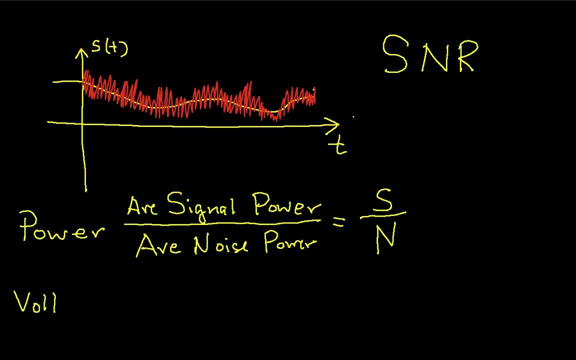 So we may have a voltage SNR Here. actually, let's change colors for this. Where this is defined as the RMS, the root mean squared signal voltage divided by the RMS. oops, got that one wrong: the RMS noise voltage. 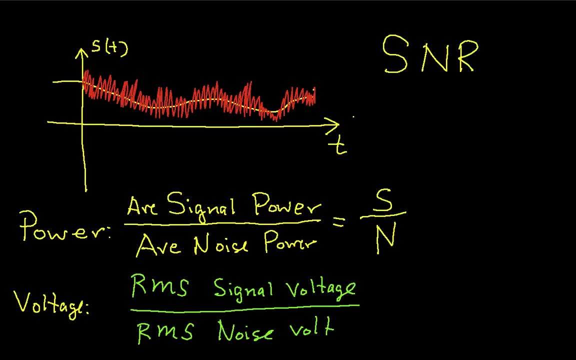 Okay. So you would expect these two to be related because, if you'll remember- or hopefully you remember either from your previous experience or a previous video- that the average signal power this guy here is given or can be computed by squaring the RMS signal voltage, 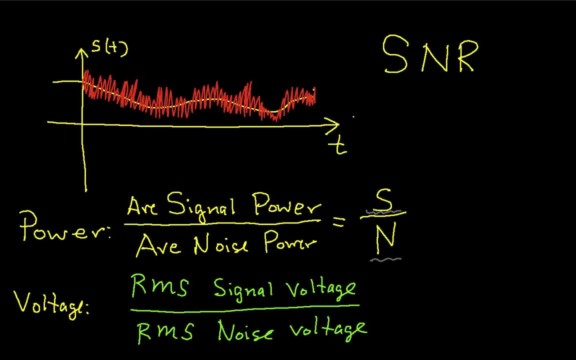 And the average noise power can be computed by squaring the RMS noise voltage. So it turns out that a signal-to-noise ratio, which is defined in terms of powers, can be expressed in terms of, oops, a signal-to-noise ratio. 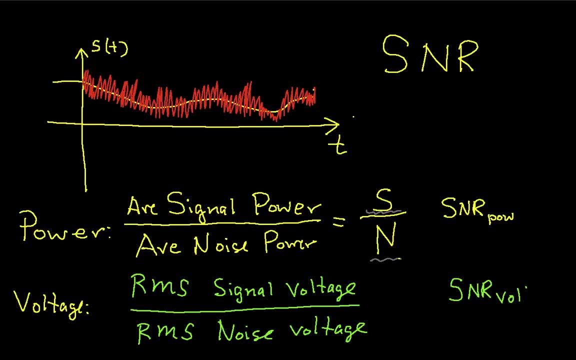 that's defined in terms of voltage as the following relationship: The power, or the power signal-to-noise ratio is the square of the voltage signal-to-noise ratio. That turns out to be quite useful. It also turns out that a very convenient way. 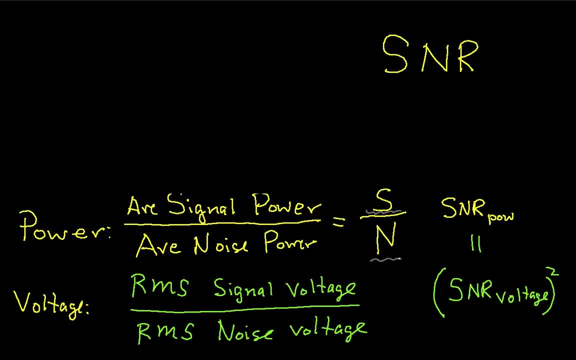 to describe a signal-to-noise ratio is in units of decibels, which are abbreviated dB, And basically, I guess I should point out, a signal-to-noise ratio is a unitless quantity because I have power in the numerator and power in the denominator. 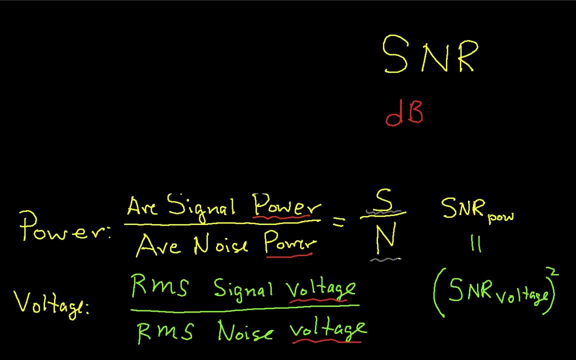 or voltage in the numerator and voltage in the denominator. So a signal-to-noise ratio is a unitless quantity. It's quite often helpful to express it in terms of dB, which is essentially a logarithmic scale. So a signal-to-noise ratio 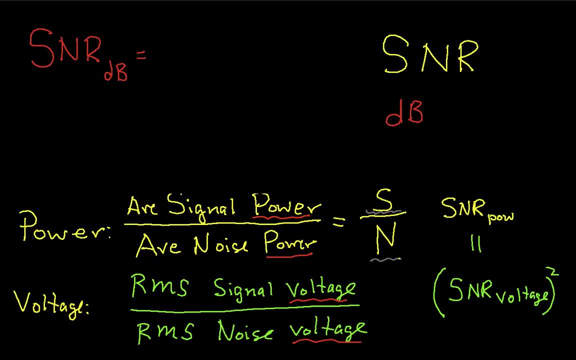 expressed in terms of dB, is given as 10 times log to the base 10 of my power signal-to-noise ratio And it's also 20 log to the base 10 of my voltage. That's the signal-to-noise ratio. 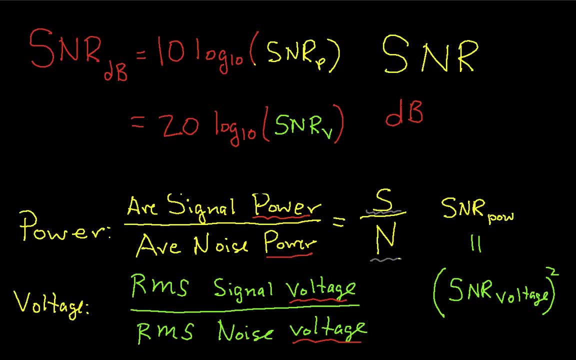 Okay, So hopefully you feel good about this, because you know that the voltage signal-to-noise ratio or, I'm sorry, you know that the power signal-to-noise ratio is obtained by squaring the voltage signal-to-noise ratio. And so because I have a log, 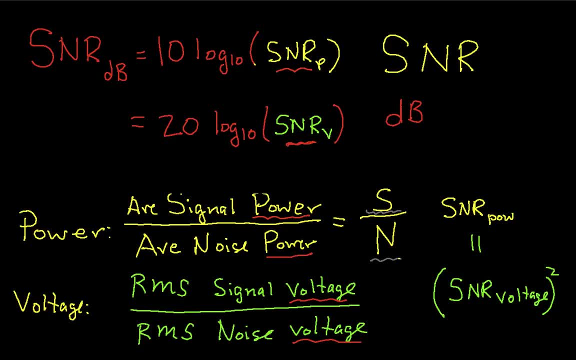 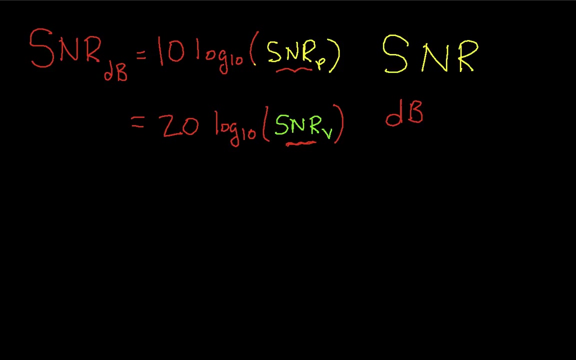 and I'm squaring things, that too comes out in front and I get basically this result: Okay, So signal-to-noise ratios are very useful. As an example of actually manipulating some signal-to-noise ratios, let's look at the following. 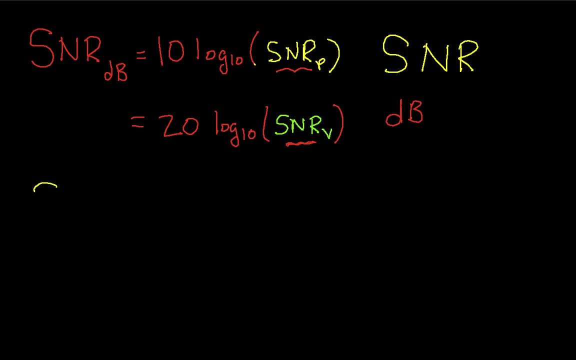 Suppose that, to begin with, my signal-to-noise ratio is 1.. Okay, So basically my noise power is the same as my signal power, And this is generally not a good thing. It means that your signal-to-noise. 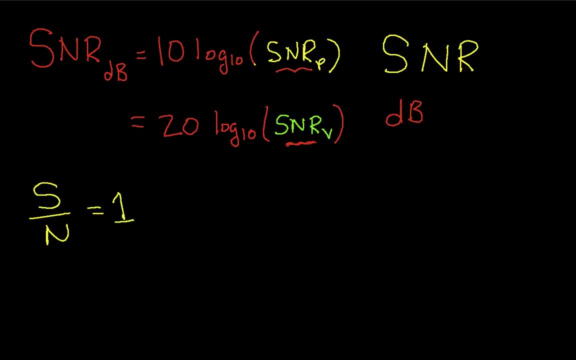 or it means that your signal is typically being swallowed up in the noise and it's very hard to get it back. If I express this in terms of dB, this is 10 log 10 of 1. log 10 of 1 is 0,. 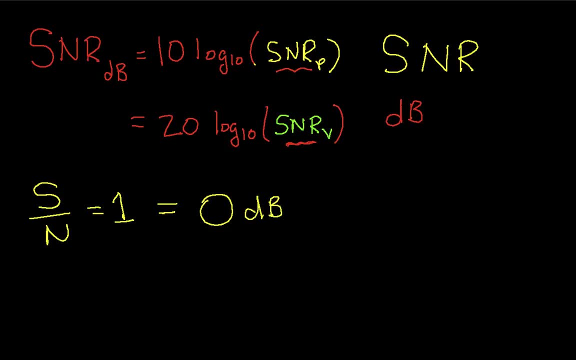 so this is 0 dB, Okay, And it turns out that this is true either for a power signal-to-noise ratio or a voltage signal-to-noise ratio, because if the ratio of the powers is 1, then the ratio of the voltages is 1 too. 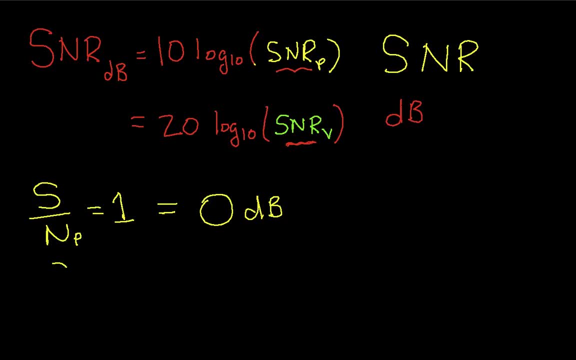 So that's sort of boring. Let's suppose then that I have a signal-to-noise ratio, a power signal-to-noise ratio of 100.. Okay, This is a much better signal-to-noise ratio, although actually not really good enough. 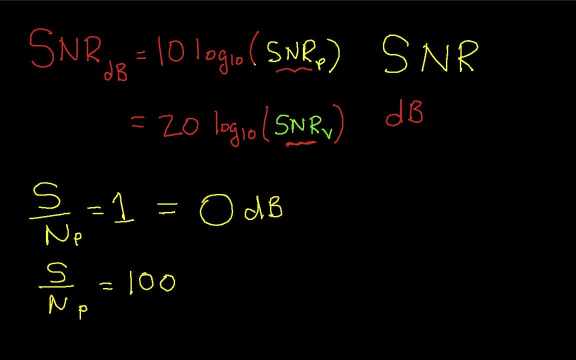 to do a lot of things that you would want to do with a signal. Okay, The voltage signal-to-noise ratio: okay. well, here actually I'm sort of mixing my metaphors here- Let's draw this guy instead as an SNRV. 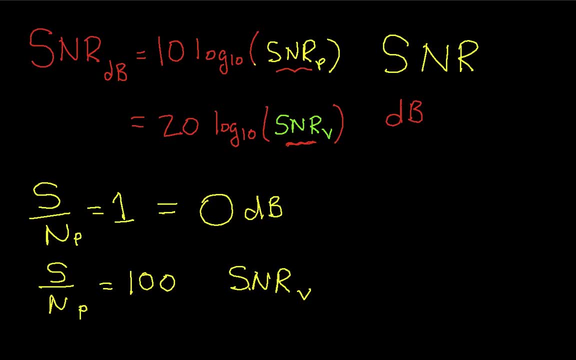 to show that this is a voltage signal-to-noise ratio. If the power signal-to-noise ratio is 100, the voltage signal-to-noise ratio is the square root of 100. Or 10.. And then, if I express this in dB: 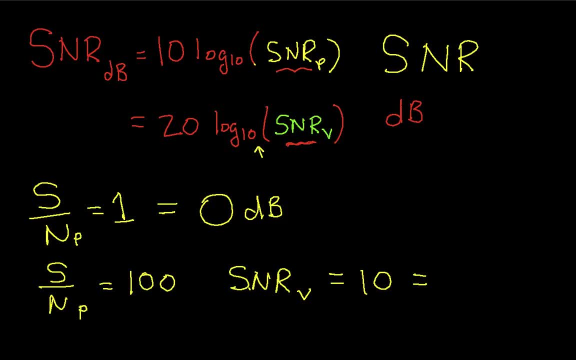 since I have a voltage signal-to-noise ratio, I'm going to have 20 log to the base 10 of 10, which is 1.. So this will just be 20 dB. Oh, I don't know what happened there. 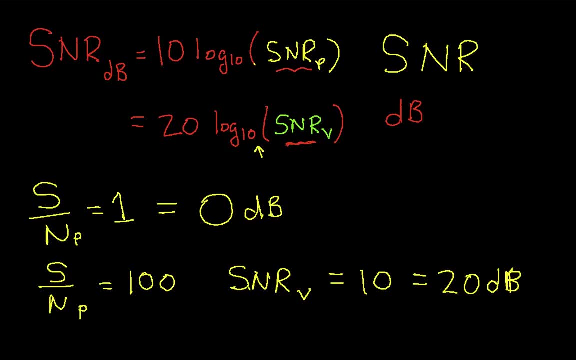 Okay, So that would give me a signal-to-noise. a power signal-to-noise ratio of 100 is 20 dB. Now I can compute this also directly, because the log base 10 of 100 is 2.. Multiply that by 10,. 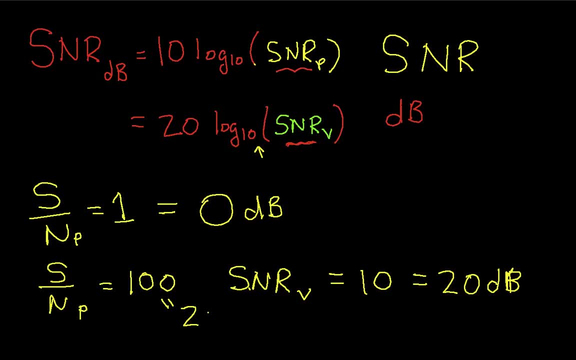 and I get 20.. So you can see that if I use dB, it doesn't matter whether I'm talking about a power or a voltage, signal-to-noise ratio. The dB expression of them is the same. So one last piece of this example. 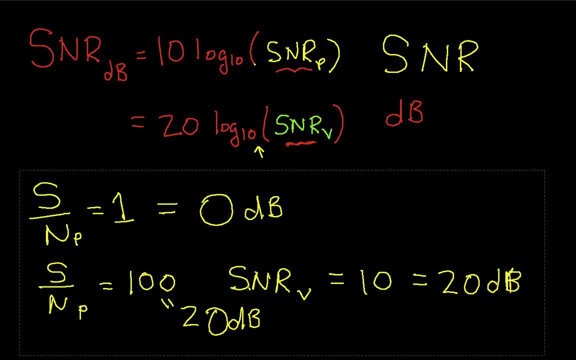 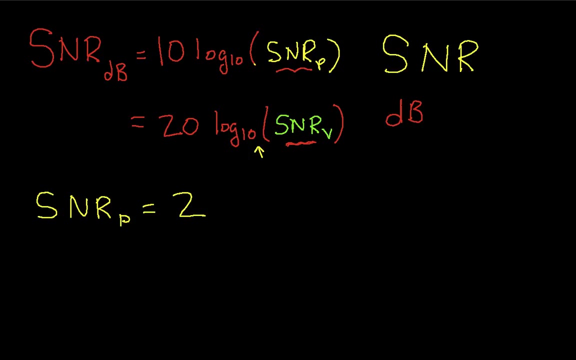 and then we'll call this done. If my signal-to-noise ratio, say power, is equal to 2, so my signal power is twice the noise power. when I express this in dB, the log to the base 10 of 2 is .301.. 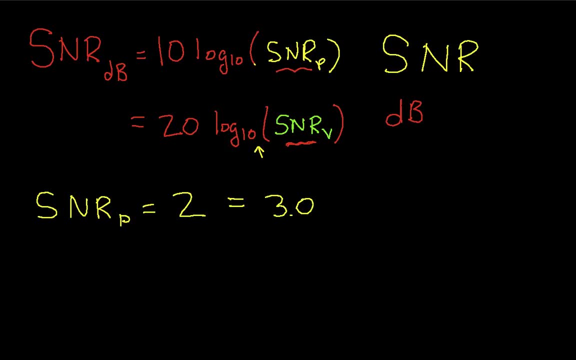 If I multiply that by 10, I get 3.01, or roughly 3 dB. I should put the dB in here too, to make sure there's no confusion. If I look at the signal-to-noise ratio- the ratio of 1 half- 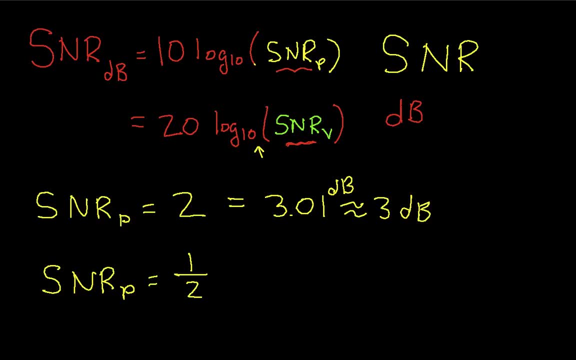 so my signal is only half as powerful as my noise. the log of 1 half, log base 10 of 1 half is minus .301.. So this then is minus .301 dB, which again is minus 3 dB. So quite often. 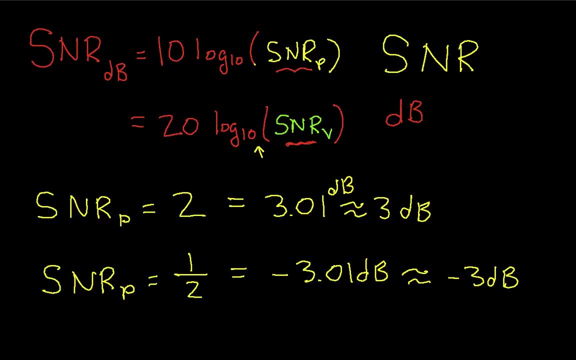 you'll see things talked about either signal-to-noise ratios or ratios of different types of powers or voltages, and you'll hear people say that I'm looking for a 3 dB gain or a minus 3 dB attenuation, or something like that. 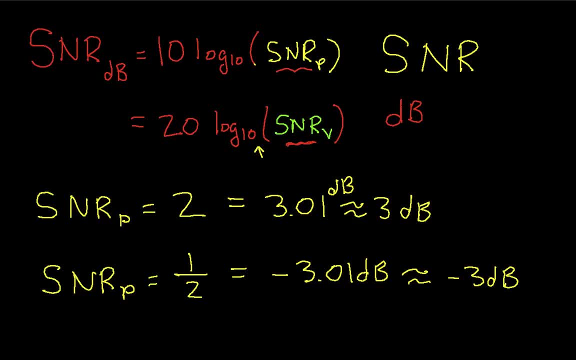 And what it means. a 3 dB gain corresponds to a ratio that's 2, so something is twice the value of something else. A minus 3 dB gain, or attenuation, means that something is half the value of something else, And so you'll see this talked about quite a bit.